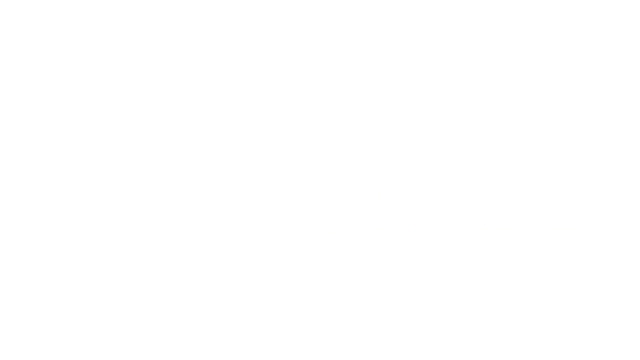 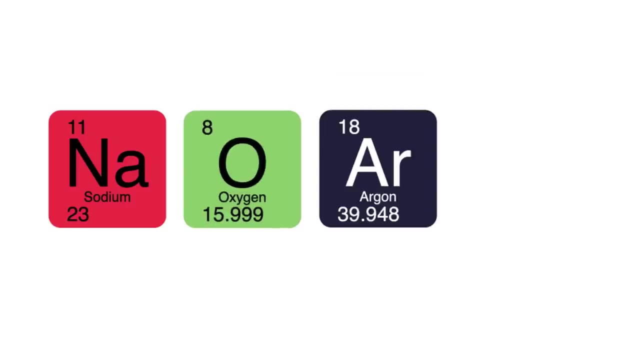 bonded together are called compounds. Each element has a different symbol, such as Na, O and Ar. What element is represented by the symbol H? H represents hydrogen. Most of the elements have symbols that start with the same letter as their name- The exceptions: 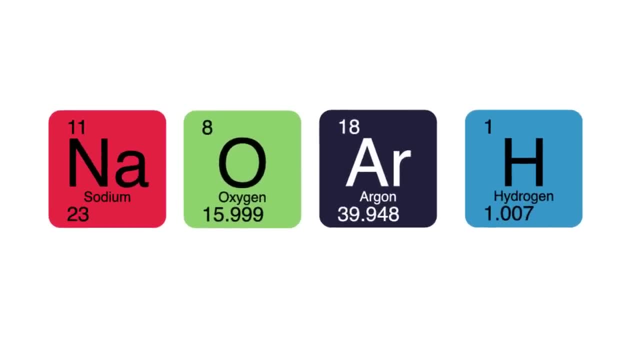 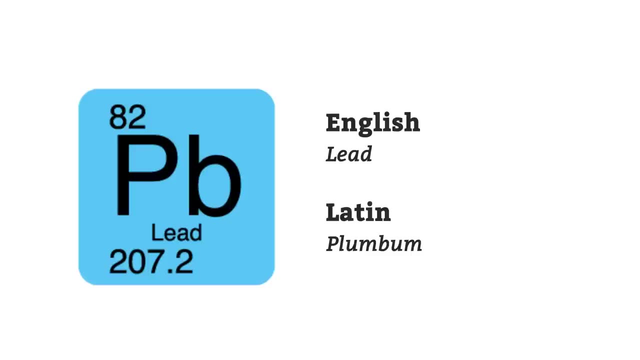 are often symbolised by a name derived from another language, like Pb for lead. This is because in Latin, lead is known as plumbum. If you look on the periodic table, you will see that the second letter of the symbol is always lower case. 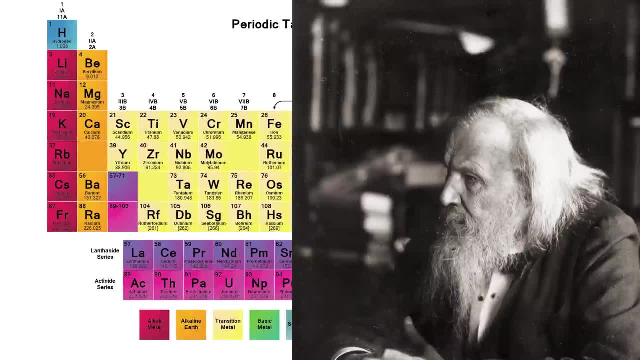 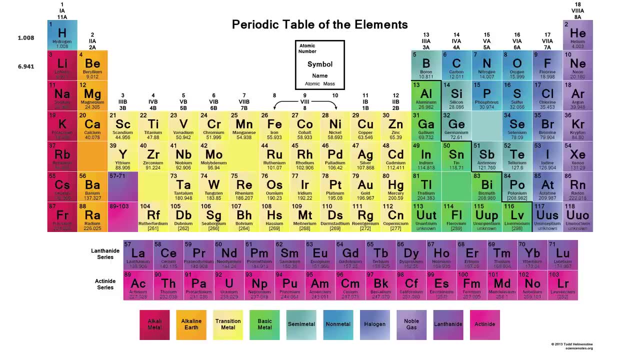 The periodic table was constructed by Dmitri Mendeleev, a Russian chemist and inventor, In 1869, he lined up all the elements in order of increasing atomic mass and then broke them into rows, so that elements with similar properties were arranged in columns. 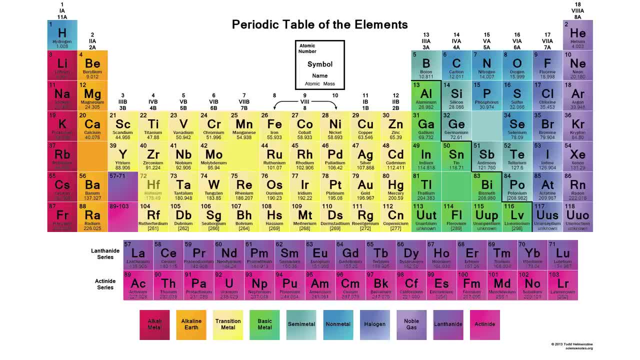 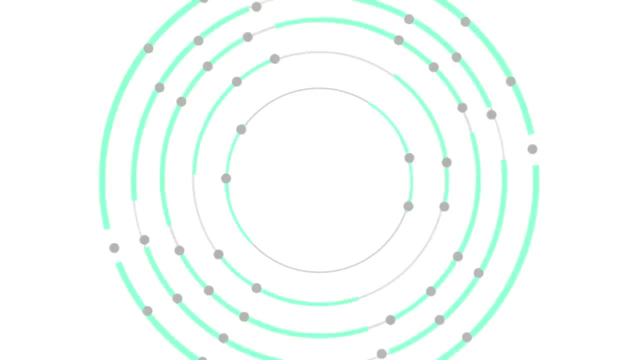 By doing this, Mendeleev was able to identify gaps and predict the properties of elements that hadn't been discovered yet. Theoretically, the periodic table could go on forever as atoms get more and more massive, But very heavy. atoms are not stable and fall apart easily. 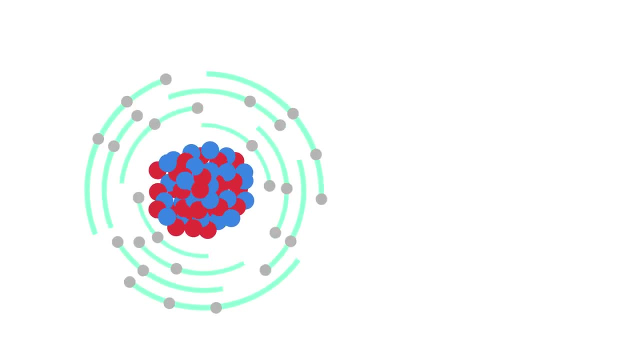 Bismuth is considered the last stable atom. This is because atoms are made up of smaller particles. What are the names of these particles? Pause the video for a moment. Atoms are made up of protons, neutrons and electrons. Protons and neutrons sit in a small central nucleus, whilst electrons orbit around the 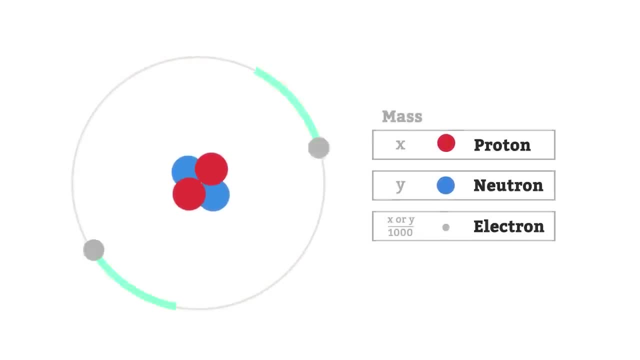 outside. The mass of an electron is about one thousandth of the mass of a neutron or proton, which means that almost all the mass of an atom is concentrated in the centre, at the nucleus, Because the mass of the proton and neutron are so much bigger than the mass of the electron. 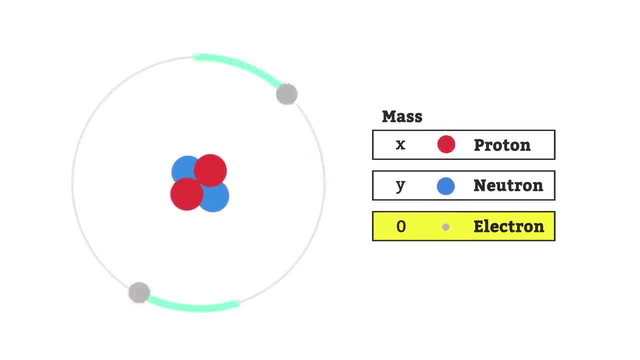 we say that the mass of the electron is essentially zero. We define elements based on how many protons they have. The number of protons cannot change. The number of protons must also be the same as the number of electrons in a neutral atom. 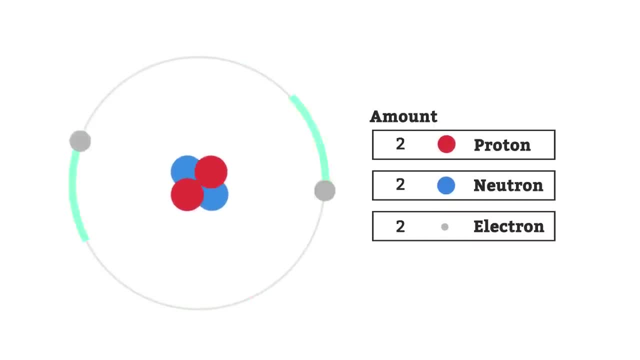 of the elements. This is because protons and electrons are charged. Protons have a positive charge plus 1, and electrons have a negative change minus 1.. If there is no difference, the atom must Changed. There are other elements as well.